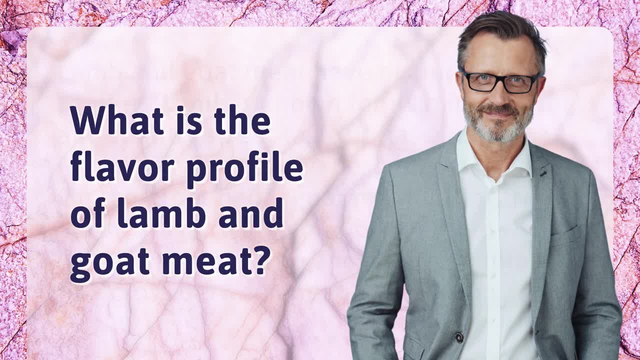 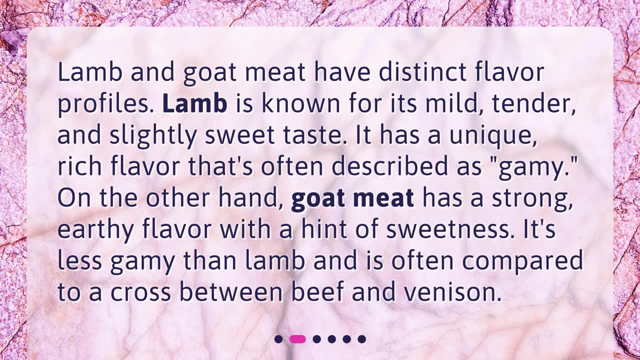 What is the flavor profile of lamb and goat meat? Lamb and goat meat have distinct flavor profiles. Lamb is known for its mild, tender and slightly sweet taste. It has a unique rich flavor that's often described as gamey. On the other hand, goat meat has a strong earthy flavor with a hint of sweetness. 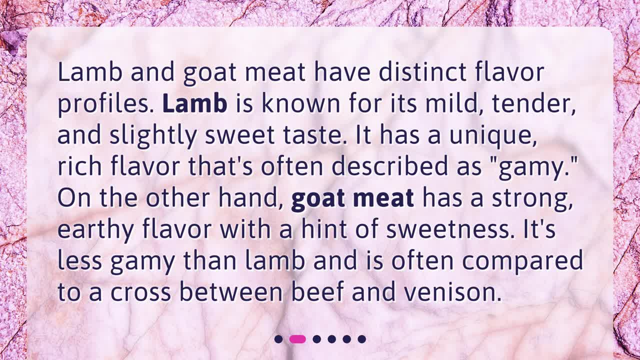 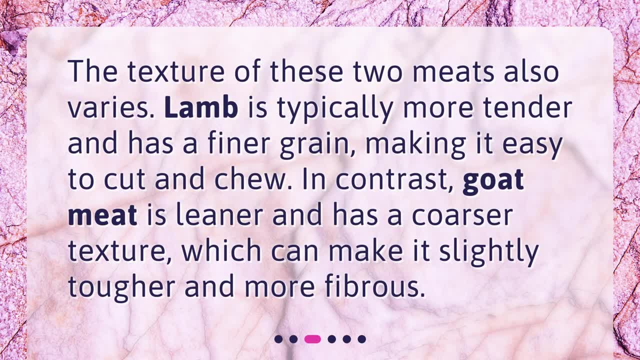 It's less gamey than lamb and is often compared to a cross between beef and venison. How does the texture of lamb and goat meat differ? The texture of these two meats also varies. Lamb is typically a meat that is cooked in a pan or a pan-fryer. 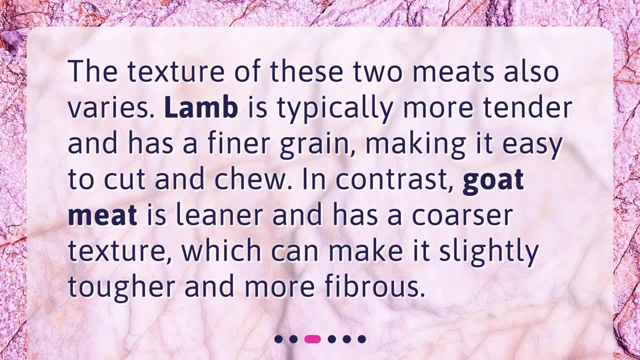 Lamb is typically a meat that is cooked in a pan-fryer Lamb is typically a meat that is cooked in a pan-fryer Lamb is typically a meat that is cooked in a pan-fryer Lamb is typically more tender and has a finer grain, making it easy to cut and chew. 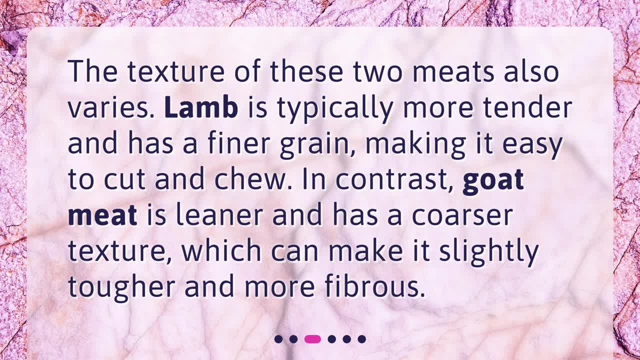 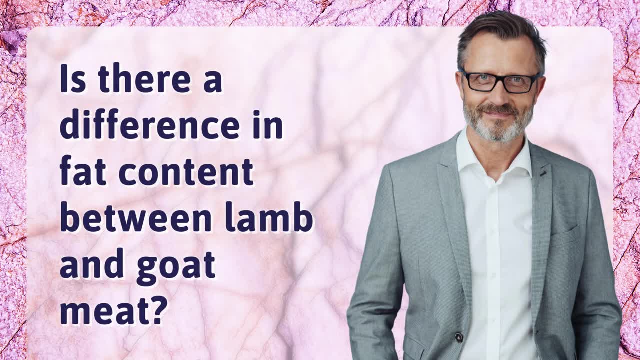 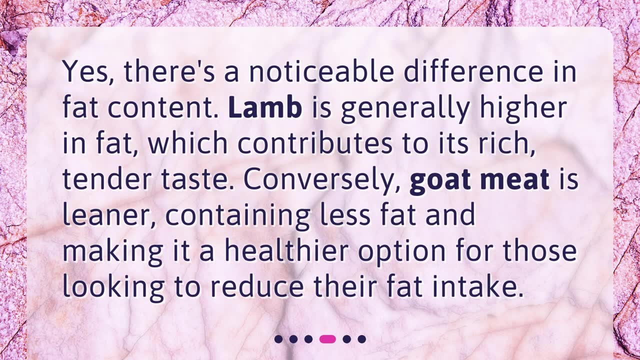 In contrast, goat meat is leaner and has a coarser texture, which can make it slightly tougher and more fibrous. Is there a difference in fat content between lamb and goat meat? Yes, there's a noticeable difference in fat content. Lamb is generally higher in fat, which contributes to its rich, tender taste. 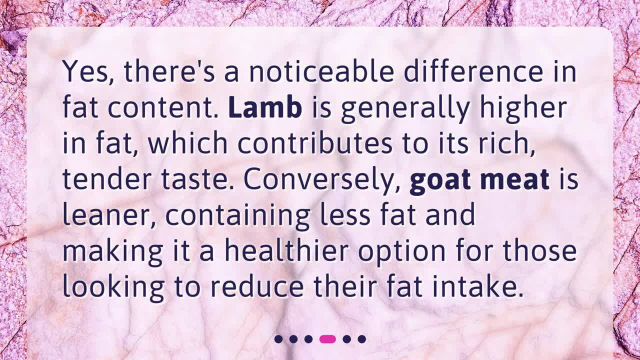 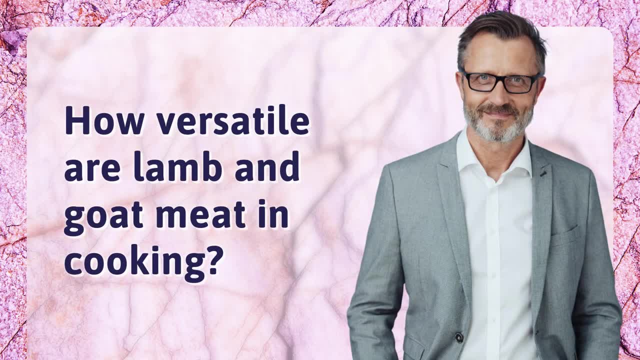 Conversely, goat meat is leaner, containing less fat and making it a healthier option for those looking to reduce their fat intake. How versatile are lamb and goat meat in cooking? Both meats are versatile and can be used in a wide range of dishes. 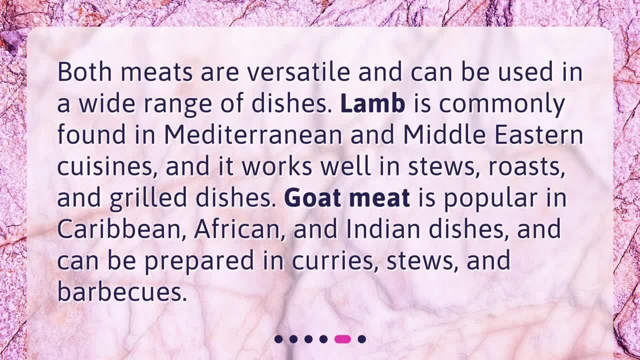 Lamb is commonly found in Mediterranean and Middle Eastern cuisines, and it works well in stews, roasts and grilled dishes. Goat meat is popular in Caribbean, African and Indian dishes and can be prepared in curries, stews and barbecues. 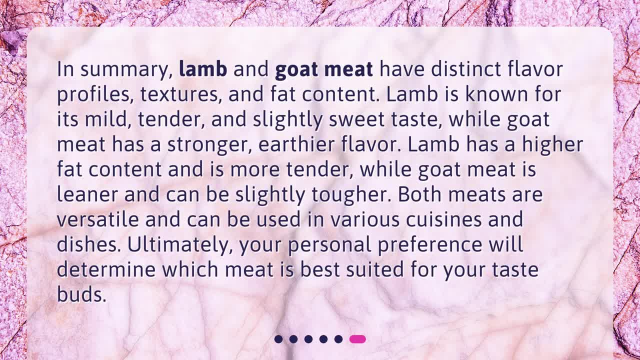 How versatile are lamb and goat meat in cooking? In summary, lamb and goat meat have distinct flavor profiles, textures and fat content. Lamb is known for its mild, tender and slightly sweet taste, while goat meat has a stronger, earthier flavor. 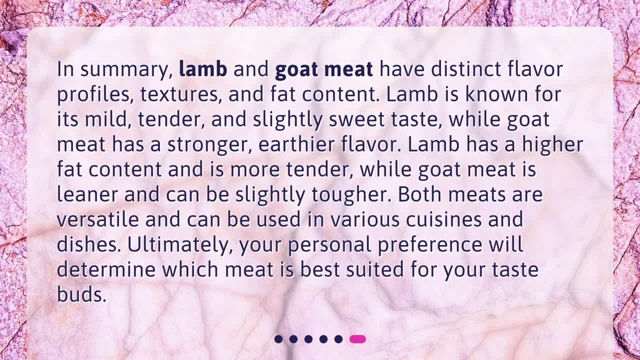 Lamb has a higher fat content and is more tender, while goat meat is leaner and can be slightly tougher. Both meats are versatile and can be used in various cuisines and dishes. Ultimately, your personal preference will determine which meat is best suited for your. 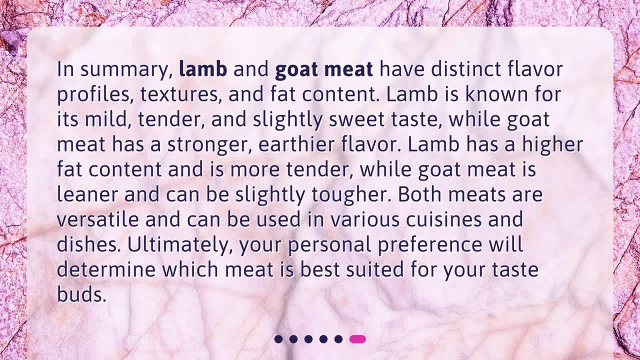 taste buds. Thank you for watching.